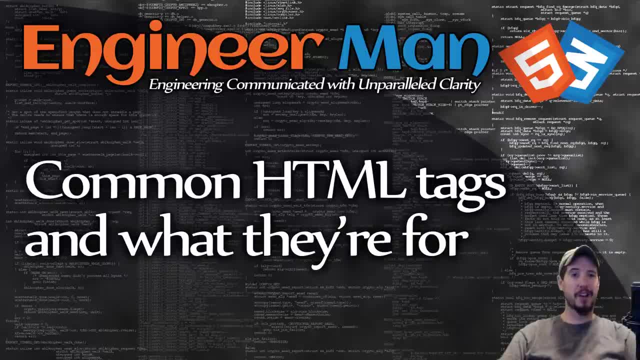 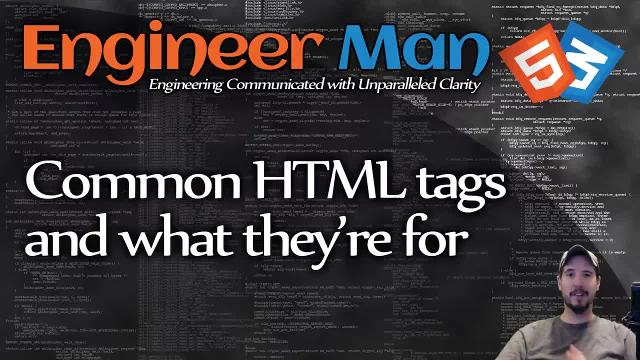 What's going on, engineers? Next on our list for HTML and CSS learnings is common HTML tags and what they're used for. For this video, we're going to take CSS. we're just going to put it aside for the most part, We're going to focus primarily on just HTML tags. Now there's somewhere around like 90 or 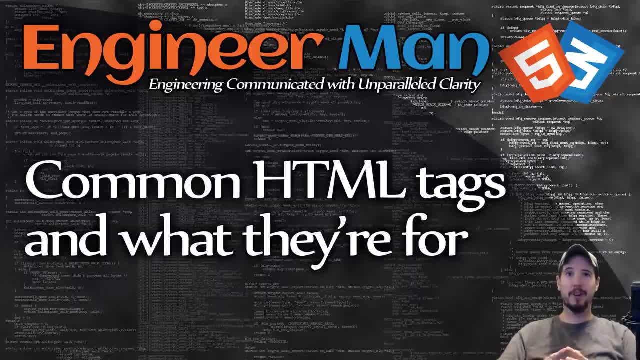 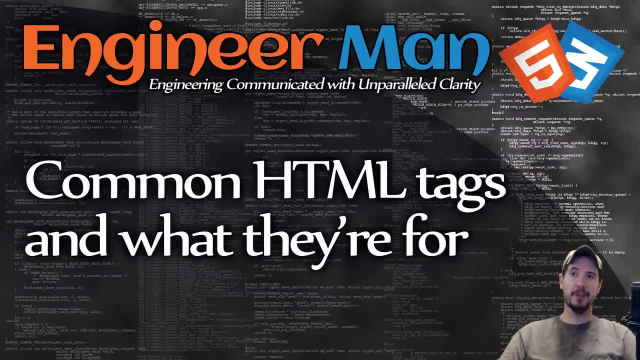 100 HTML tags in total, but we're not going to look at all of them today. We're going to look at about 15 of the most common ones For most websites. about 90% of the tags that are used you're going to see in this video. So let's get started. In the first HTML and CSS video I did, we talked about 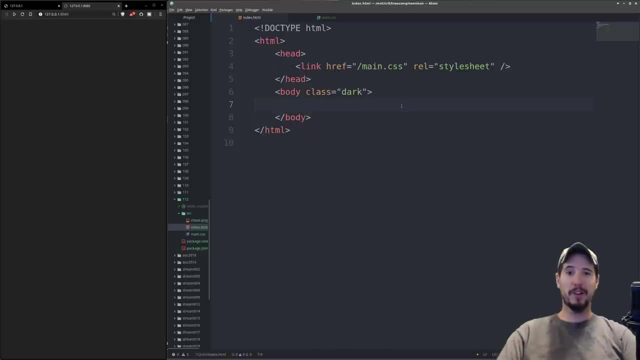 what HTML and CSS was for, and we talked about what a minimal document would look like, So we're going to start with that same document for this video, which is a simple HTML tag. Inside of that, a head and body tag. I am including a small CSS file, but you can ignore that entirely. Its only. 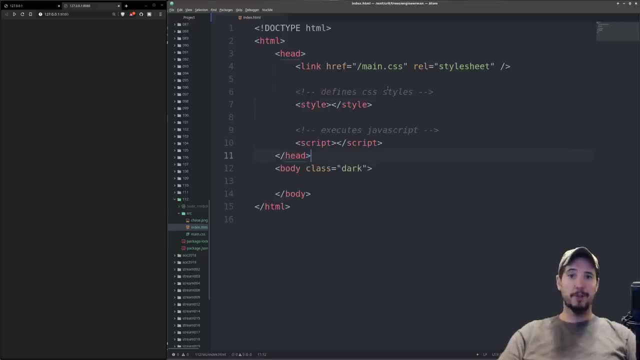 purpose is just to make what we're making dark theme. The first two tags we're going to look at are the style and script tags. and these two tags: they are typically located inside of the head tag, but it's not strictly required. You can put them in the body tag as well if you wanted The style. 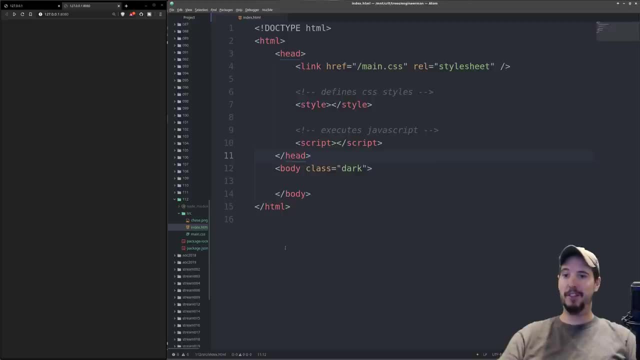 tag is used for defining style and script tags. The style tag is used for defining style and script tags. It can be used in lieu of a CSS file. If I wanted to, I could go into maincss. I could copy and paste all the styles out of it and into the style tag, and it would have the exact same effect. As far 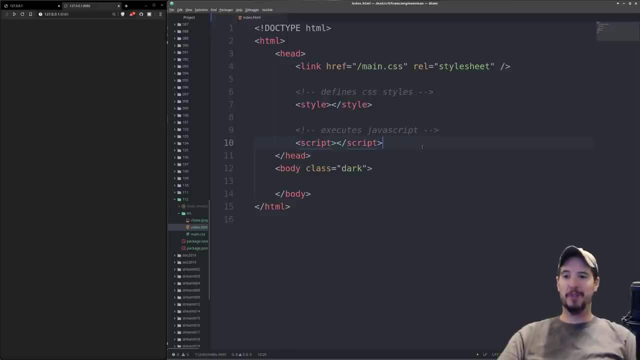 as the script tag. it works the exact same way as the style tag, except it's for JavaScript. Instead of including a JavaScript file, if you wanted to just include your code directly into your HTML document, you could include it between script tags and it would execute as soon as it got to it. 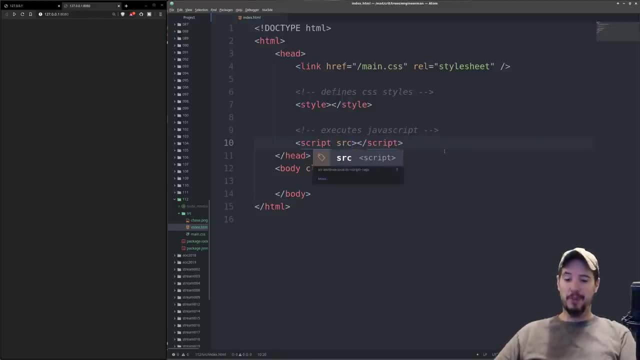 However, if you wanted to include JavaScript from a file, you can simply do a source attribute and specify the name of the file, and then that will import it. For the remaining tags, they're all related to the actual rendering of visual aspects in the browser and that means we're going to put them all inside the body tag, The first I want to look. 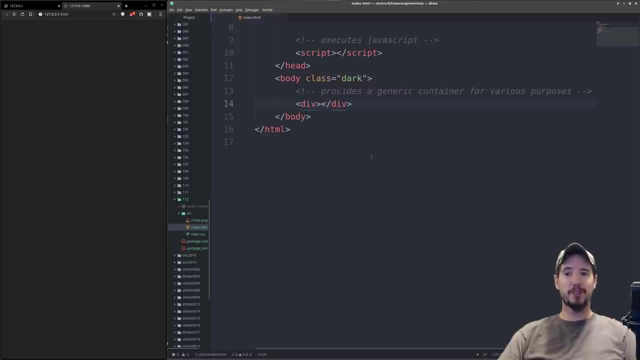 at is the div tag, and the diff tag can be thought of as the most common generic container for various purposes, whether that's text or other elements. What the div ultimately looks like is based entirely on how you style it. Of course, we haven't styled it at all here, however, because 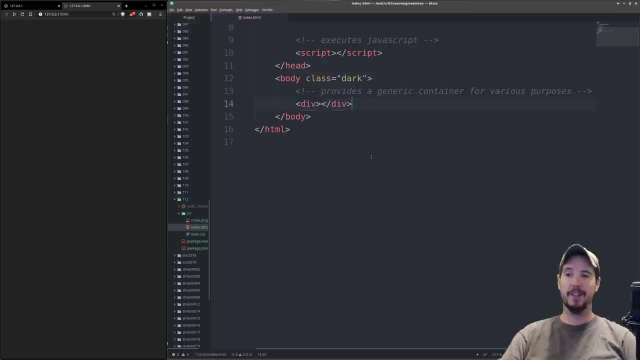 each tag has implied styles. that is, the browser will look at the tag and say, okay, well, I don't see anything styled here, so I'm going to apply a certain style to it. The div and a couple tags we're going to look at after this are what's called block level elements, which means by default they. 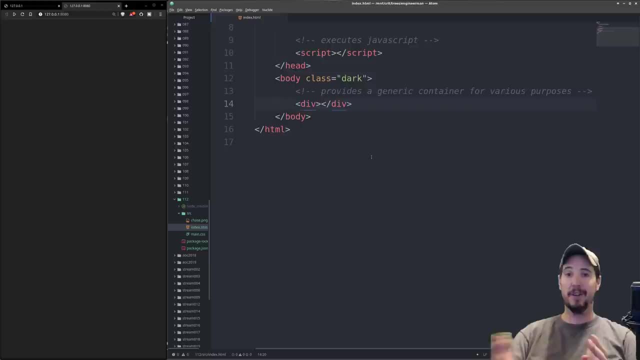 are 100% wide, filling the either parent element or the screen in this case, and their height is just going to be whatever the height of the content is. Just so you can visualize what this element looks like, I briefly added a CSS style to it to make the background red, and you can see over here. 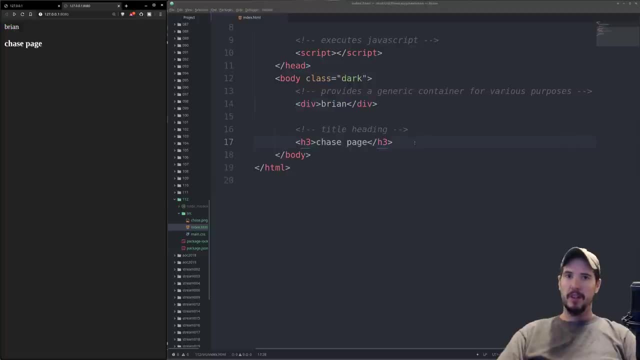 it's 100% wide and it contains text inside it. Next tag we're going to look at is for title headings, and it's going to be h1 through h6, a total of six tags. Now, like a div, this is a block level. 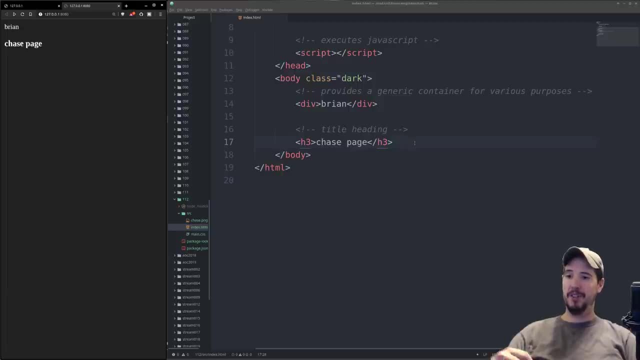 element, but the browser is going to give it top and bottom margin and then it's going to give it a small or large size, depending on whether it's h1 through h6. So an h1, of course, is going to be the largest- We can see that here text is quite large- and then h6 is going to be the smallest. So you, 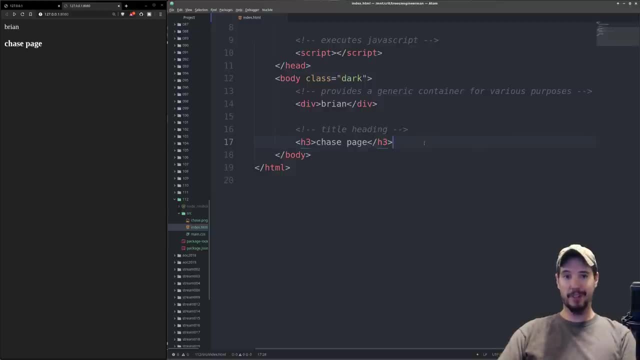 might be thinking to yourself: well, how come I can't just take a title text, put it in a div, and then I can't just take a title text and put it in a div, and then I can't just take a title text and make it larger and make it bold? and the answer is: you absolutely can. The reason you want to: 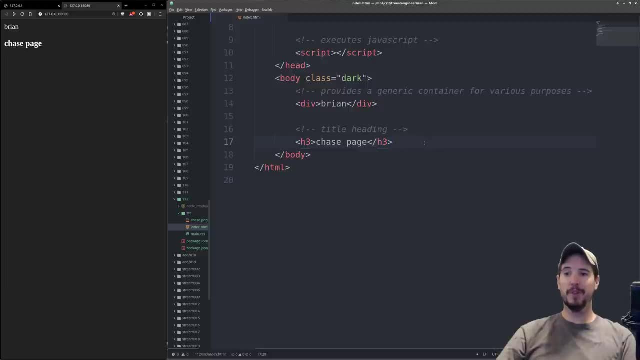 prefer an h3 or an h4 tag over a div is because it's not enough to just make your website look properly. you also want it to be semantically accurate in the way it's structured. For instance, programs that read html will know that an h1 through h6 is supposed to be a title, irrespective. 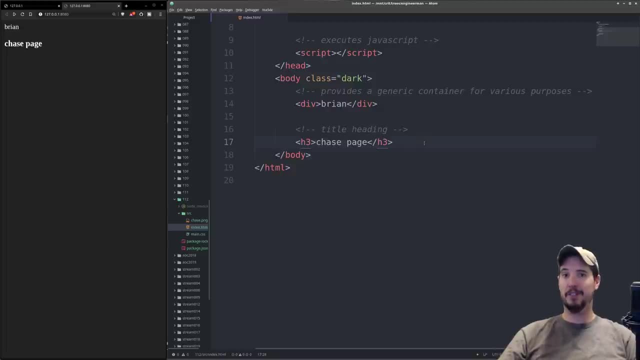 of whether or not it's styled to look like one, Whereas a div that's styled to look like a title will still just be a div. Next tag is a p tag and it stands for paragraph. This tag is intended to contain blocks of text, and here again you could use a div for this. but if 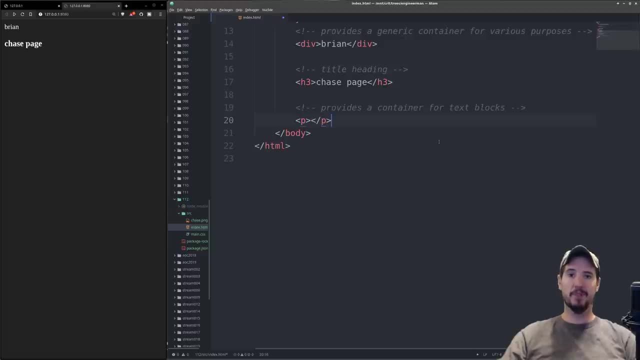 you have a block of text, using the p tag is going to be more semantically accurate. The next tag is the br tag, which will insert a line break, And the reason the br tag is even necessary in the first place is because, by default, html trims all trailing and leading white space and then 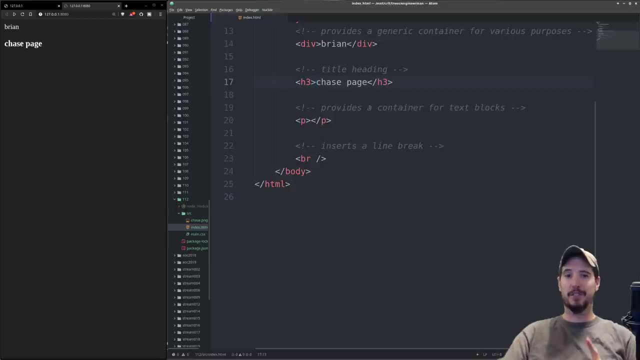 all sequences of white space between elements are seen as one single space. So let's look back at the h3 tag again. So if I have chase page here, if I put a bunch of spaces between the elements here, it's actually the exact same content. You can see. it doesn't change on the right If I insert: 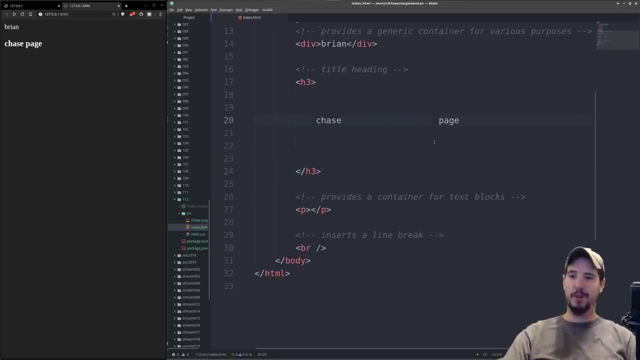 additional spaces here. same thing again. it doesn't change If I put this on a separate thing here. indent it out, it's all the same text. We'll use a br tag in a little bit and it'll make more sense. The next tag is a span tag and the span tag is most common you use for wrapping inline elements. 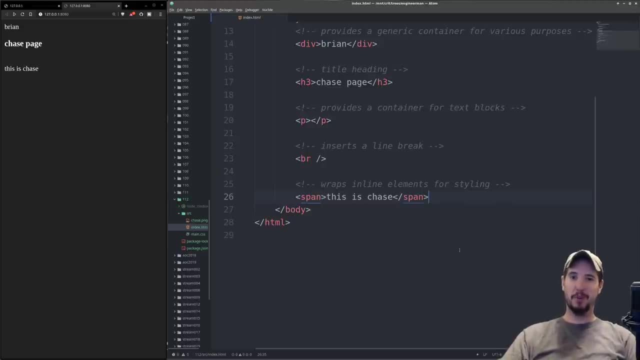 for styling. So imagine you had a block of text and you wanted just a couple words to be bold. You could wrap just those two words in a span tag and then make them bold. Next tag we're going to look at is for showing an image on the screen. Now, this is the first visual tag that we need to. 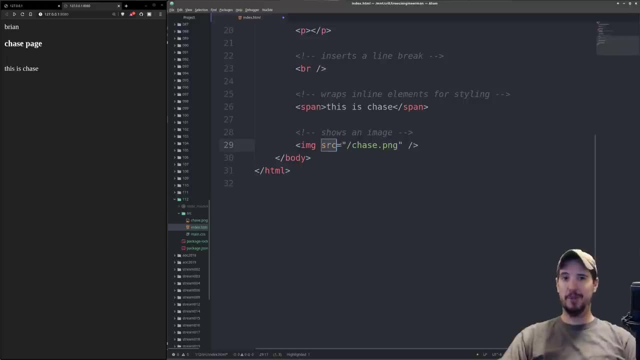 actually use a specific attribute, and this is the src attribute, which stands for source, and then you'll supply where that image is on the server. And, of course, when I save my document, then the picture shows up on the screen. But note what happened here: it took the text I had and then 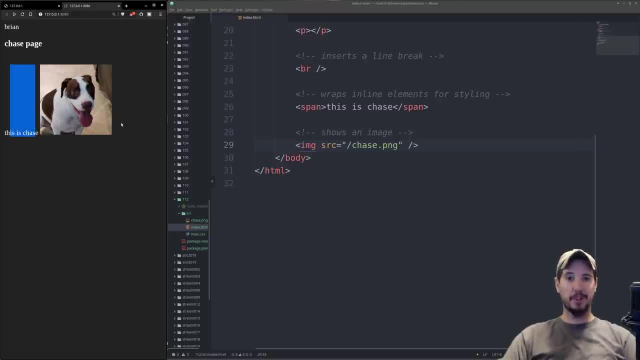 add the image directly to the right of it. Now, remember, I said we're going to use the br for something real well, this is what it is. So, because these are two inline elements, if I want to get the text I have to add a br right here and then, once I save it, then it goes below it Until I add that. 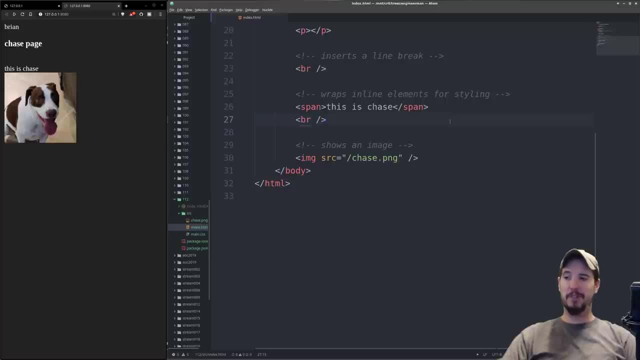 br, all HTML did was just ignore all the white space and all the new lines, and it just put the two things next to one another. The next I will look at is an, a tag which stands for anchor, and this tag is for creating hyperlinks which can allow you to link to other pages. So the a tag does take one. 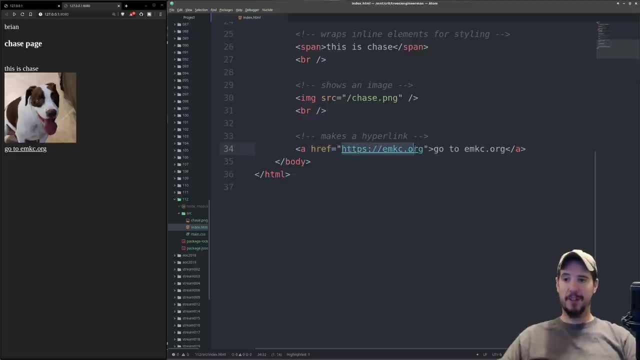 attribute called href and then in the href you supply the site they should go to when the link is clicked, And then inside the a tag you'd specify the text that should actually be displayed on the screen And you'll notice the browser added this underscore. I did not add this. 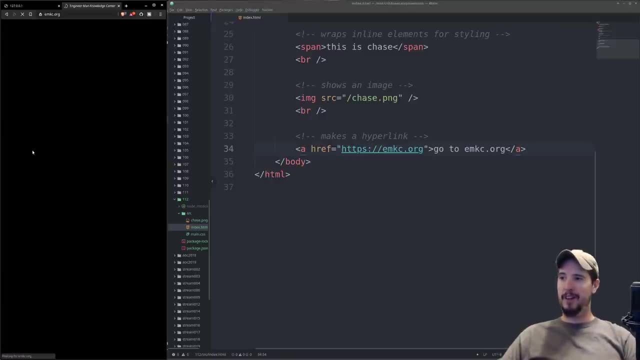 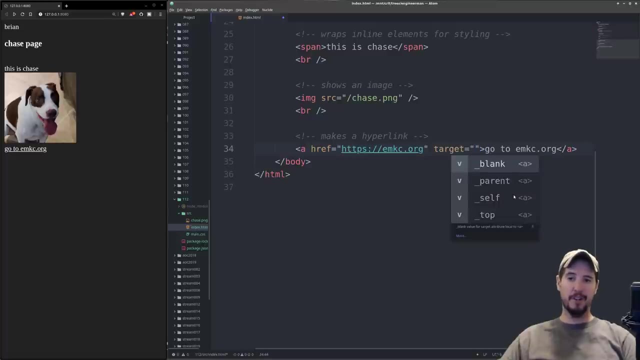 this is just a browser default. And then, of course, when I click on the link, it navigates me away to emkcorg. If you want to make it so, the link opened up in a different tab. there's a second attribute you can use, called target, and then from the options you can select blank. And then now, if 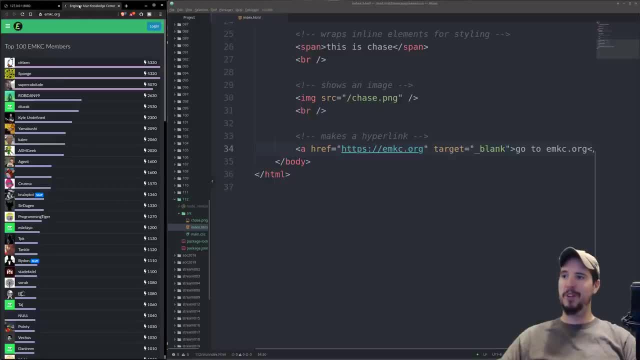 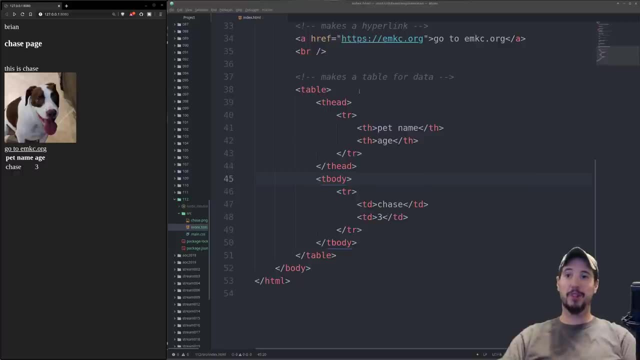 I refresh the page and I click the link, you can see it opens up in a brand new tab, as opposed to navigating away. Next tag is the table tag, which is for doing tabular data, think like rows and columns. So the tag table has two tags inside it. it has a t head and a t body tag. Inside the t head tag is: 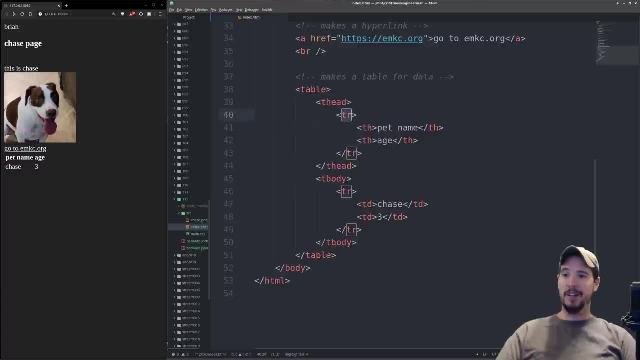 the tr tag, which is table row, and inside the table row tag is two th tags which stand for table header and this is designed just for the first row which typically shows the column header name. so like pet name and age and over here you can see it here: pet name and age Inside the t body we again have 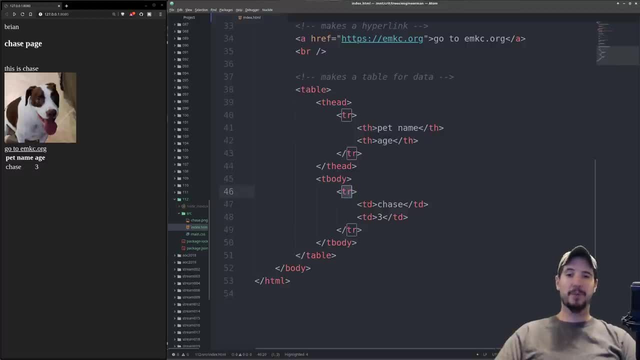 another tr table row and inside this we have td tags, which is table data. So for the first cell I have a pet name and for the second cell I have three which goes below age, and if you wanted to add additional rows, all you would do is just copy and paste the tr tag and you can see over here now. 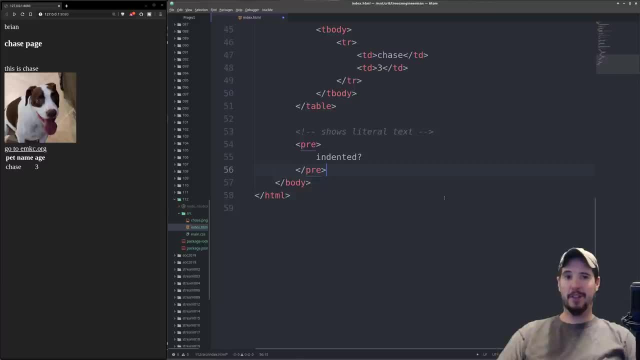 I have three rows. The next tag is the pre tag, and you remember earlier when I said the HTML completely ignores whitespace and none of that matters. well, the pre tag is the one exception. Whatever is inside the pre tag, which stands for pre-formatted text, will show exactly on the screen, as you have. 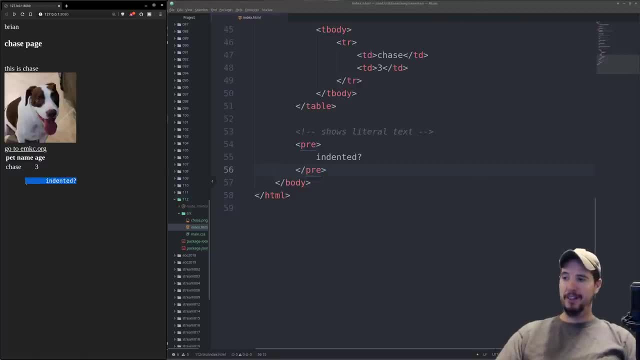 it written. As you can see over here, the word indented is in fact indented out and it's indented in the exact amount that is here in the document. The other thing this does is prevents wrapping. Ordinarily, when you type text, it will wrap when the screen gets too big for the text, but in the 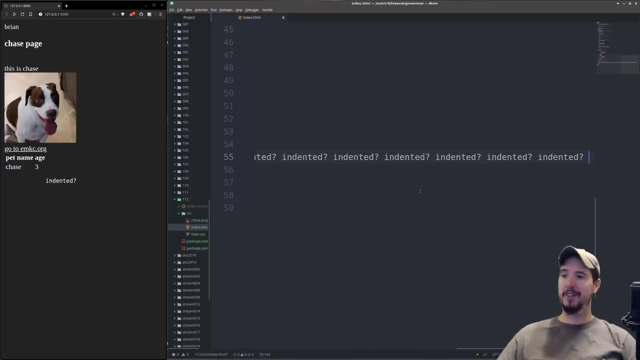 case of the pre tag. if I take this and I add a bunch of data after it and I click save, you can see that now it gives me the scroll bar and I have to actually scroll out to get to it all. It doesn't wrap to the next line. it's actually showing literally what you've written. This is different. 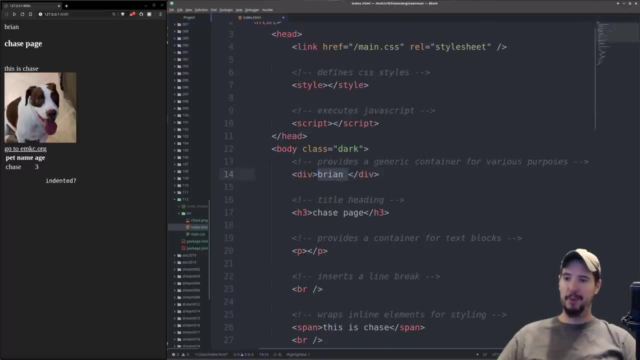 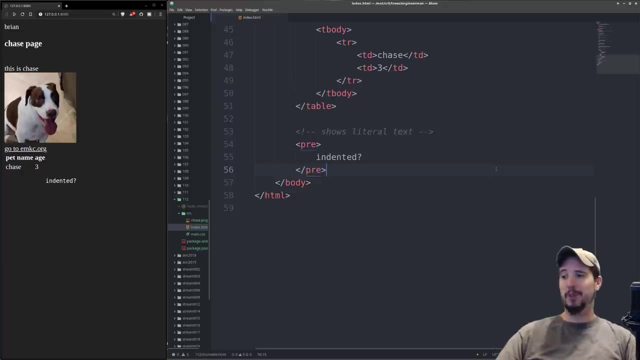 of course, than if I came up here to my original div- and I copy and pasted this a bunch of times. you can see that once the text gets too big, then it wraps. So the remaining tags we're going to be looking at all deal with the user actually giving input onto the screen, things like text boxes and buttons, and so 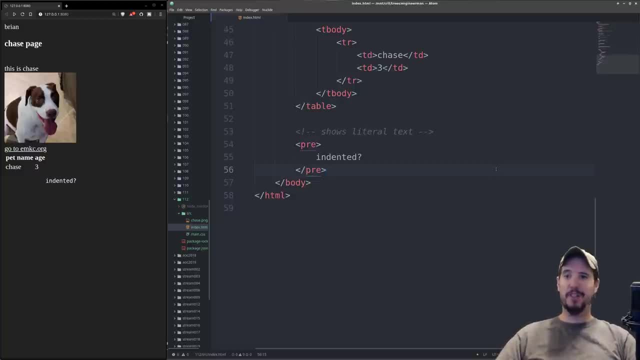 on The tags that we've looked at so far. if used with sufficient complexity and enough CSS, you can pretty much make any site any way you want. In future videos, now that we know how each tag works, we're going to look at actually composing sites with HTML. The first user input tag is going 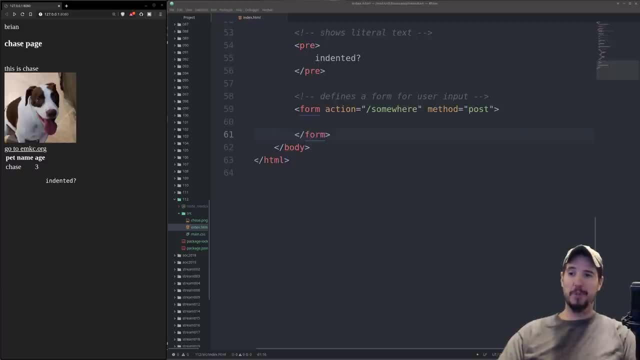 to be the form tag, and typically the form tag will wrap a bunch of input elements. The form tag, when compared with a submit button, allows the posting of data to a various endpoint on a server. How exactly the back end reads and processes it, of course is out of the scope of this video, but do 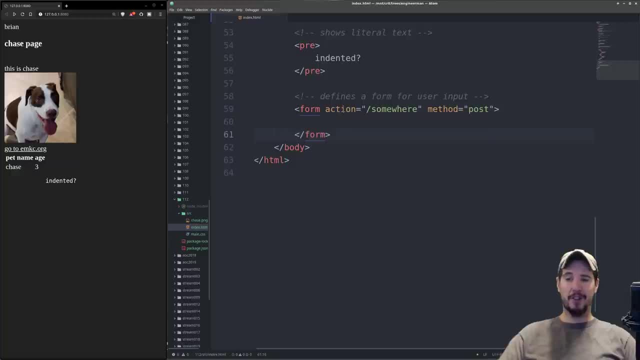 know that for a form tag, you have two attributes. primarily, you have the action, which will be the URL it should post the data to, and then the method will be the HTTP verb that should do typically get or post. The first info we're going to look at is just a simple text input. This is going to 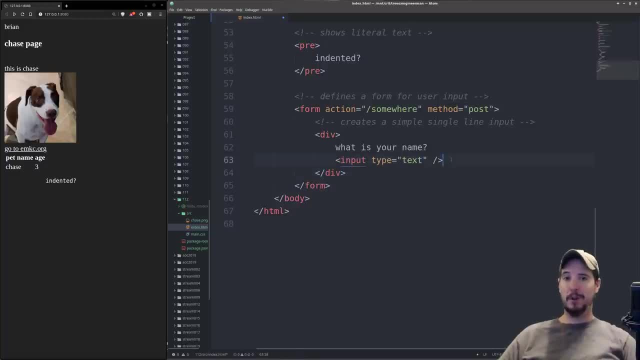 input tag with a type equals text. now note that i wrapped this in a div. i'm doing this because all the inputs are all inline elements, meaning that they'll all just stack on top of each other. so by using a div, this will allow each one to go on a new line. so if i save this, we look over here. 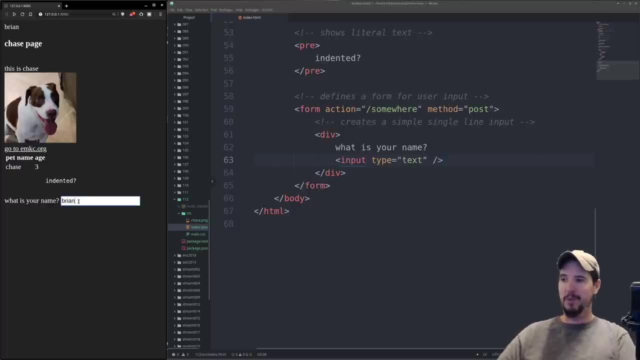 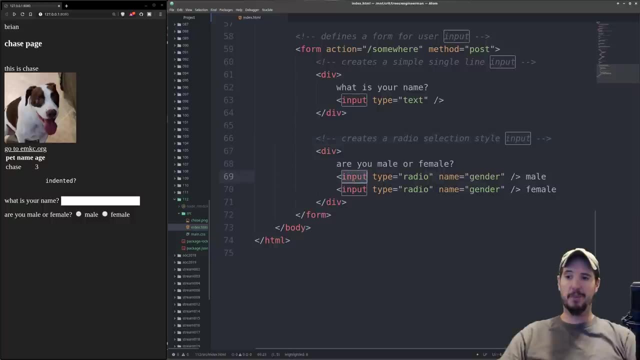 we now have a label called what is your name and we have a box that we can type some name or whatever. the next input type we're going to look at is a radio input type, and you'll note that the tag is actually the same. they're both input, it's just the type has changed. so in this case it's. type radio. now, one of the specific ways that the radio buttons work is that it can have either nothing checked, or you can check one or the other. you're not allowed to check both, and that functionality is provided by the browser. as long as you name the two radio buttons the same, then. 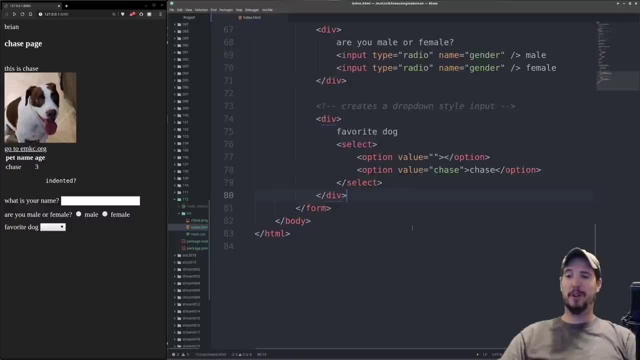 the browser will take care of the rest. the next input type is just a drop down list of options. now, this is a different tag. this is going to be a select tag, and then inside the select tag is one or more option tags. now the option tag takes a value attribute as well as something between the 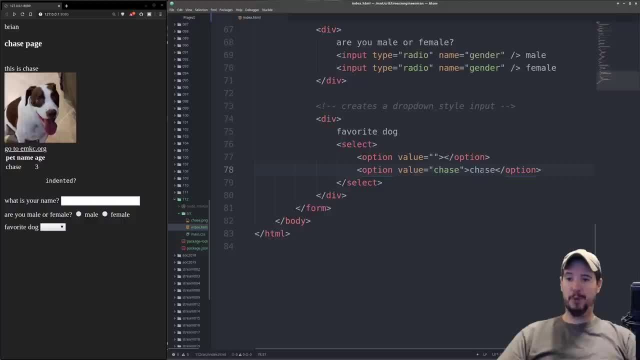 tag itself, and there's a subtle difference between the tag and the option tag, and the option tag is going to be the text that's actually shown in the drop down itself. however, the text that's in the value attribute is going to be the thing that's sent to the server if you were to post this form. 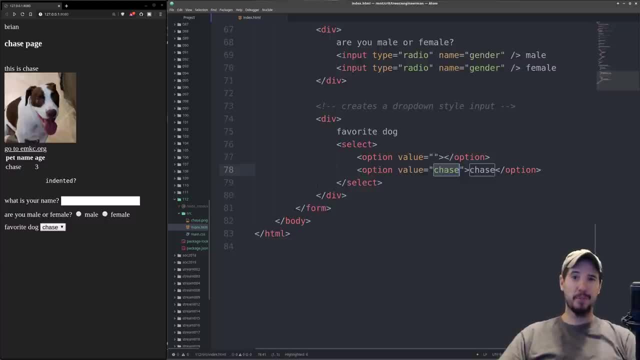 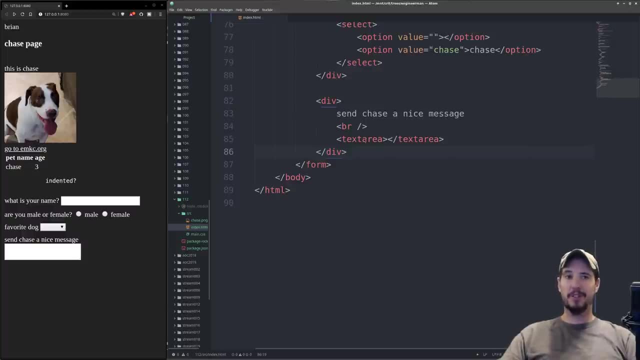 to a server. in many cases, both the value and the text is the same, but not always. now the next input is called a text area, and this is a lot like a text input, with the exception of a text area can be multiple lines, and then it's also resizable in the browser by default, and then if you type text, 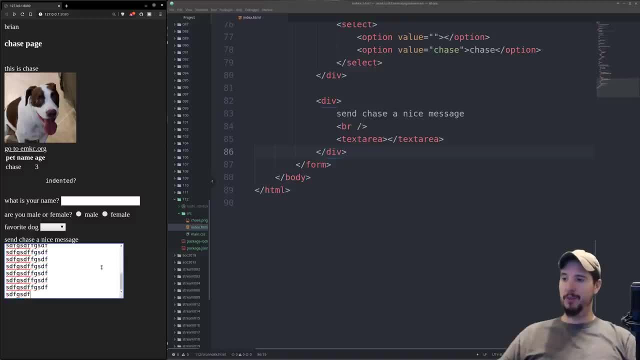 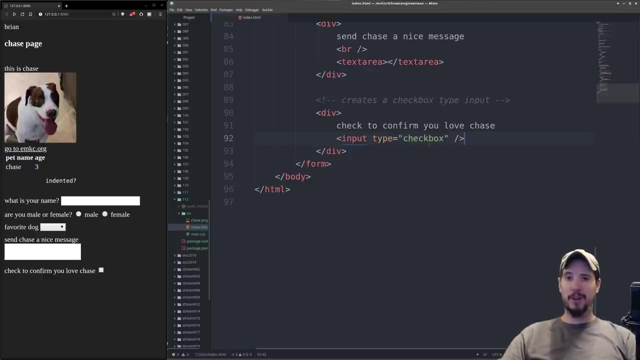 that's beyond the text area. it's going to be the text that's actually shown in the drop down itself. and then the last input type is an input type check box, and this is going to make a checkbox that can be either checked or not checked. this differs from radio buttons in that if you have 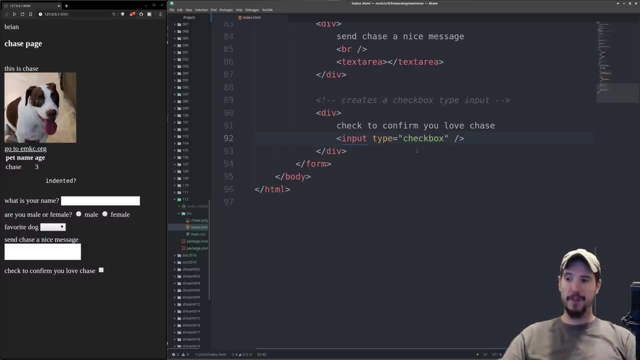 10 check boxes. you can check either zero of them, you can check all of them, half of them, it doesn't matter. so use check boxes if you want people to select zero or more of something, and use radio buttons if you want somebody to select typically exactly one thing. and then, finally, the last.